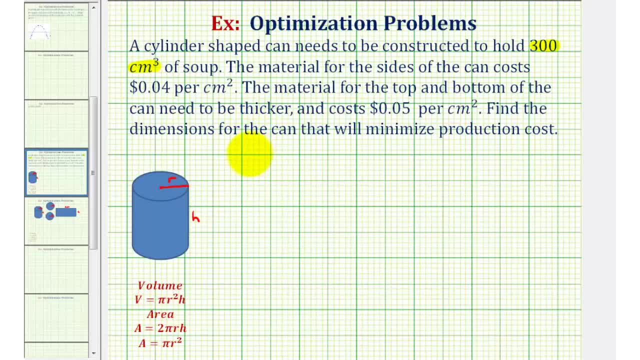 is equal to pi r squared h. for this problem, pi r squared h must equal 300 cubic centimeters. This is called the constraint. Next, the cost function involves the surface area of the cylinder, as well as different costs for the top bottom. 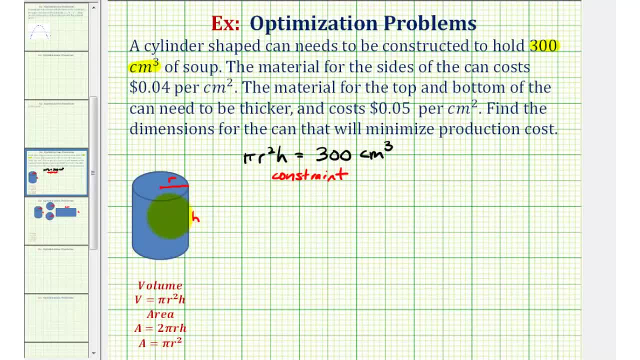 and side of the can. So let's first talk about the surface area of our cylinder. If you can imagine cutting out the top and bottom of the can and then slicing the side and unrolling the side, hopefully you can visualize that it would look something like this: 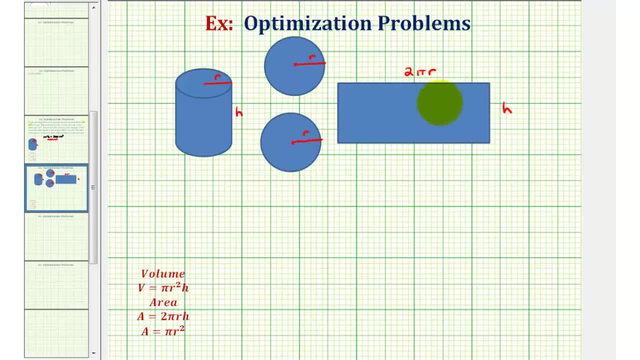 where this would be the top and the bottom and this would be the side of the can. Notice how the radius for the two circles and the cylinder would be the same. The height of the can would give us this length of the rectangle, And then this length. here is a little tricky. 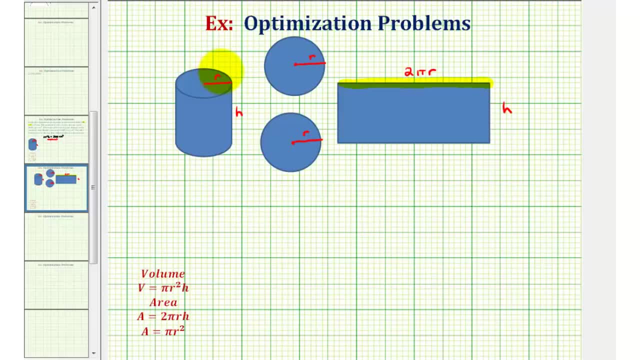 This actually comes from the circumference of the circle here And the force of the force here. the formula for the circumference of a circle is equal to two pi r And again, remember, the cost for the top and bottom is five cents per square centimeter. 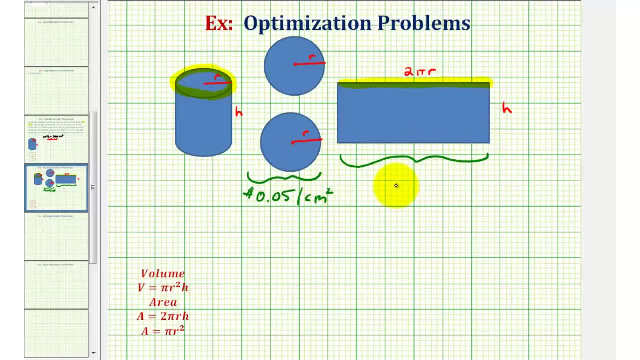 And the cost for the side is four cents per square centimeter. So with this information we can write the cost equation. The cost is going to be equal to five cents times the area of the two circles. times the area of the two circles. 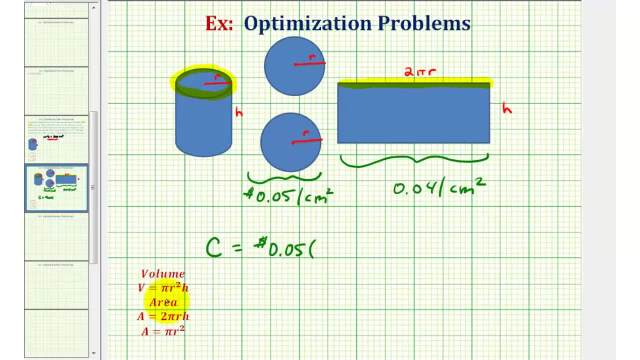 times the area of the two circles. Well, the area of a circle is equal to pi r squared. so we'd have times two pi r squared, plus four cents times the area of the rectangle, which would be two pi r h. So let's go ahead and take this cost equation. 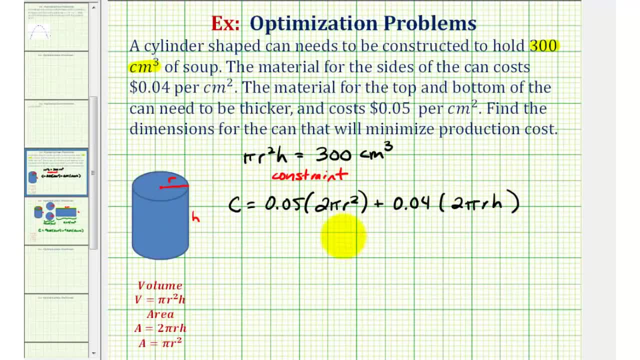 back to the previous slide. Remember: our goal here is to minimize the cost, but we want the cost function in terms of one variable. but we want the cost function in terms of one variable and right now it's in terms of two variables. 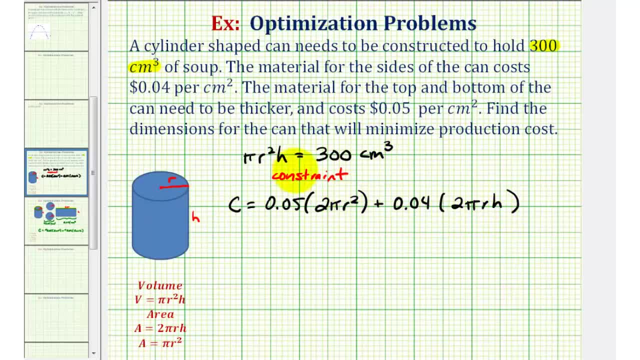 both r and h. So what we'll do now is use the constraint to perform a substitution so that we can obtain the cost function in terms of just r. To do this, we're going to solve the constraint for h, so we're going to divide both sides of this equation. 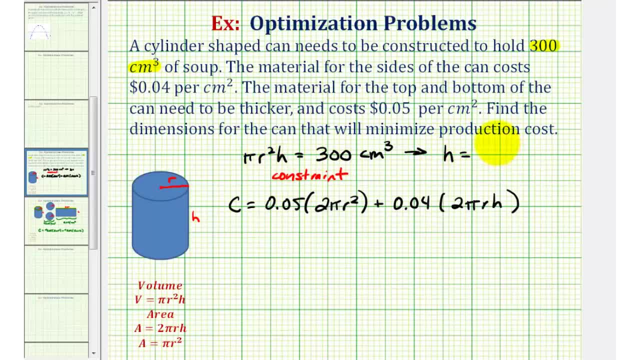 by pi r squared. so h is equal to 300 divided by pi r squared. Now we can substitute this quotient here for h in our cost equation, So we would have c equals 0.05 times two is 0.1, so we have 0.1 pi r squared plus 0.04 times two would be. 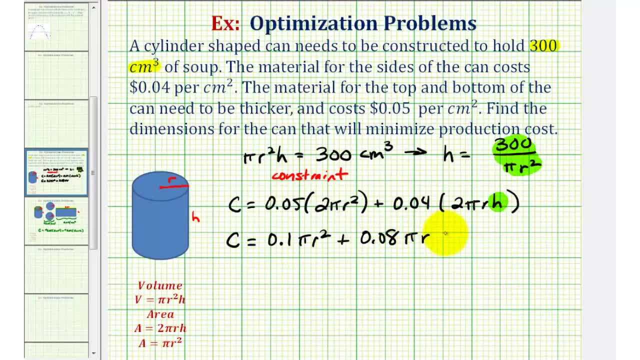 0.08 pi times r times h. but again, h is equal to 300 divided by pi r squared. Now let's go ahead and simplify this product here. Pi over pi would simplify. to one notice: one factor of r would simplify as well. 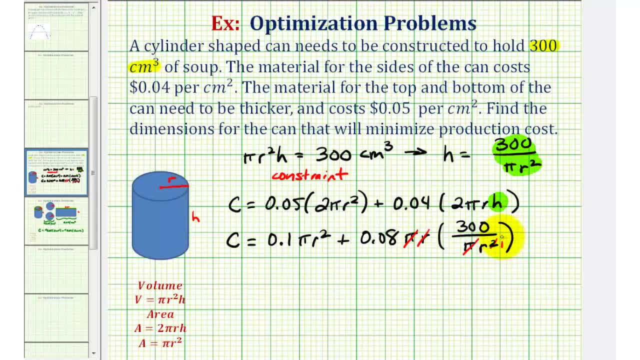 This would simplify to one. this would simplify to r to the first. So now we have the cost function in terms of r. We have: c equals 0.1 pi. r squared plus 0.08 times 300 is 24, so we have 24 divided by r. 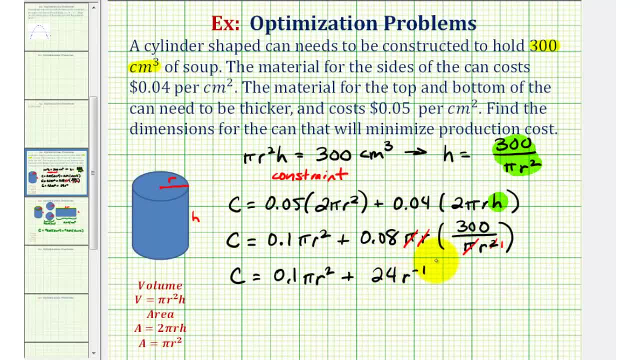 which we can also write as 24 r to the power of negative one. Remember, if we move r up into the numerator or across the fraction bar, it's going to change the sign of the exponent. So now that we have our cost function in terms of r. 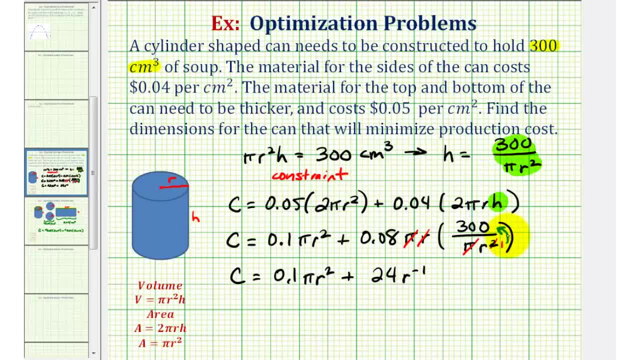 to minimize c. we'll find the critical numbers by determining where the first derivative is equal to zero or undefined, and then from there we'll determine which value of r minimizes the cost, So c prime which will be the derivative with respect to r. 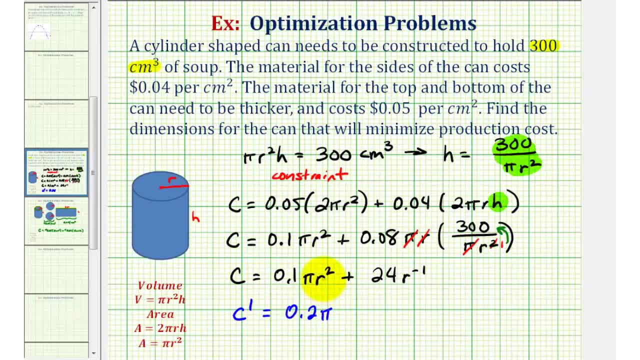 would be 0.2 pi times r to the first, or just r, and here we're going to multiply by negative one, so we'll have minus 24 r to the power of negative one, minus one or negative two. Let's go ahead and take this derivative function. 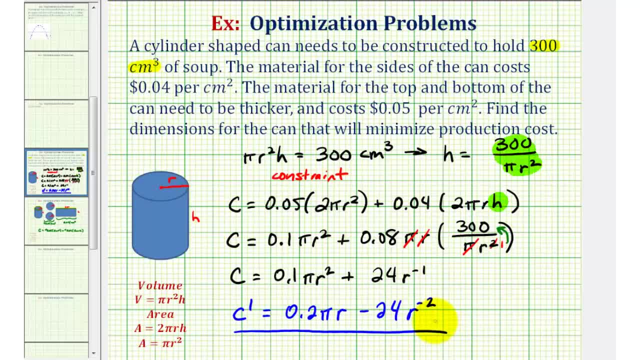 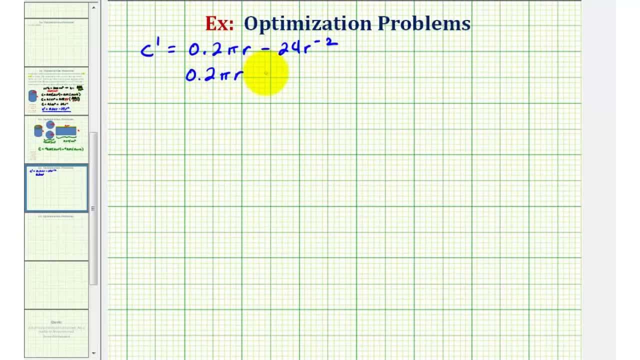 to the next slide to determine where it's undefined or equal to zero. Let's go ahead and rewrite this as a fraction. We can write this as: 0.2 pi r minus 24, divided by r squared, equals zero. Now we can see it's going to be undefined. 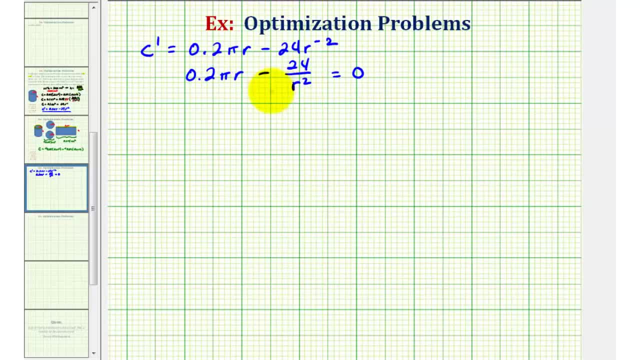 when r equals zero. but we know the radius can't equal zero. therefore we'll just go ahead and solve this for r by multiplying both sides of the equation by r squared. So on the left side we're going to have 0.2 pi r cubed. 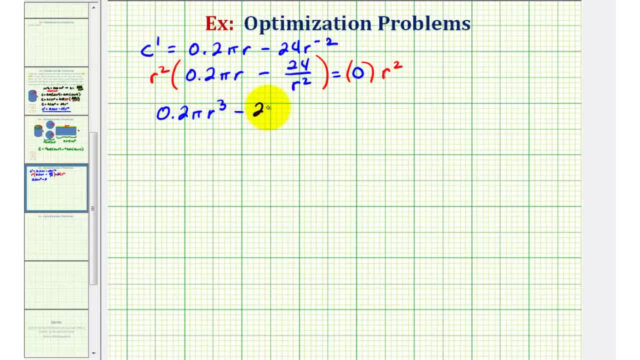 Notice how the r squareds will simplify out. so we'll have: minus 24 equals zero. We'll go ahead and solve this for r cubed, so we'll add 24 to both sides And go ahead and divide by 0.2 pi. 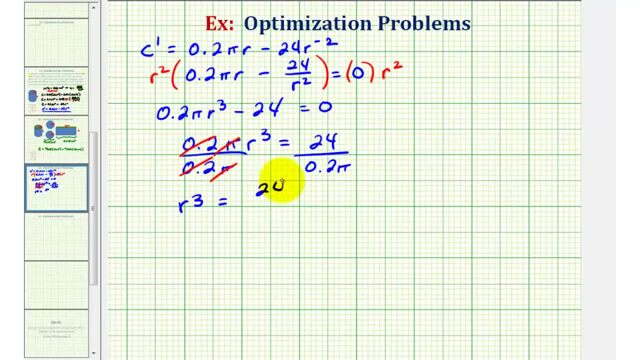 So we have r cubed equals 24 divided by 0.2 pi. Now to solve for r, we'll take the cube root of both sides of the equation. To save some time, I've already determined this value. We have r's approximately equal to three point three six. 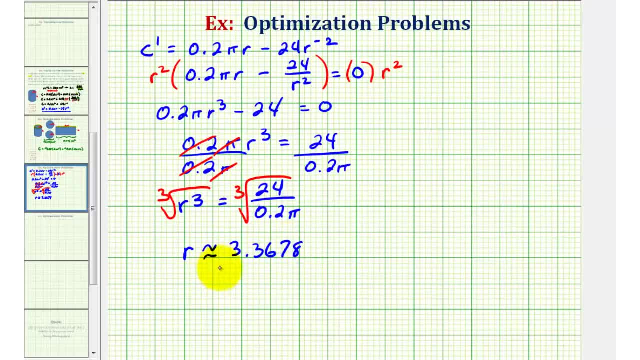 minus 24.2. pi six, seven, eight. Now, because we only have one critical number, we probably would be okay by assuming this value of r is going to minimize the production cost. but just to be sure we should use either the first. 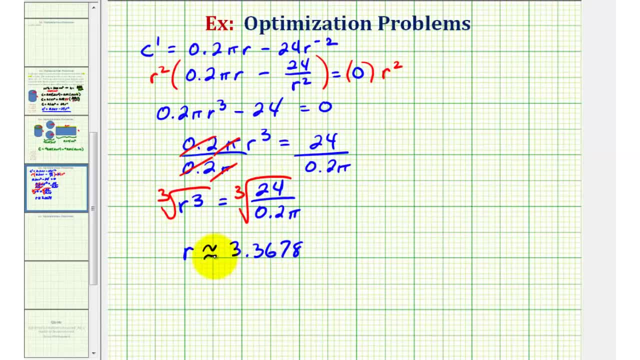 or second derivative test to make sure we do have a minimum value at this value of r, Let's go ahead and use the second derivative test. So if here's the first derivative, then we can find the second derivative To find the power rule. here we would just have 0.2 pi. 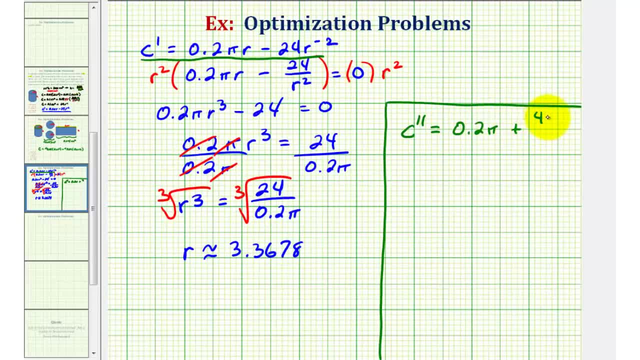 Then we multiply it by negative two, so that's going to be plus 48 times r to the power of negative three, which is the same as dividing by r to the third. Now notice if we substituted 3.3678 for r. 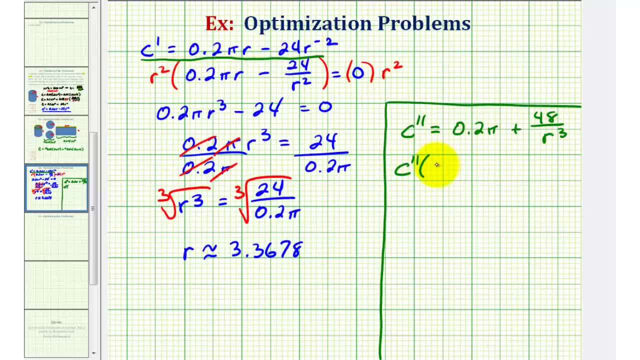 this sum would be positive. so c double prime of 3.3678 would be greater than zero, which means the function would be concave up, which is good news, because if the function is concave up at this critical number, that means we'd have: 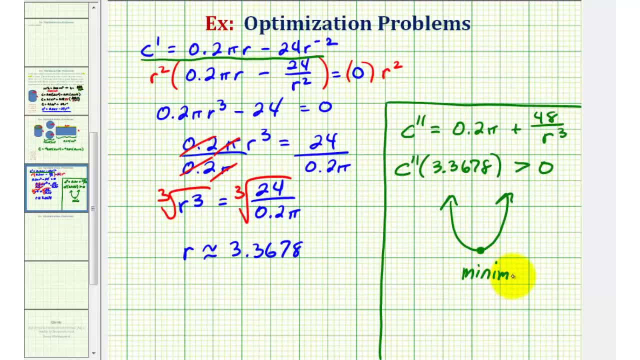 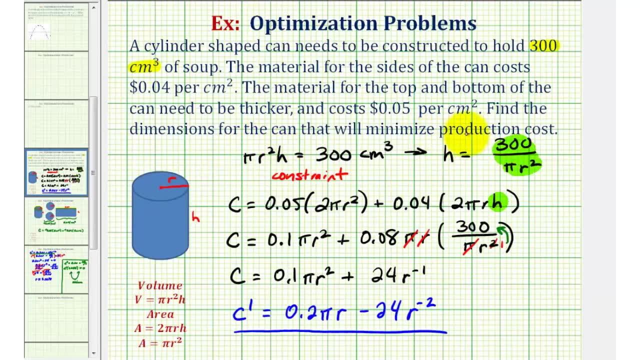 a minimum function value or, in this case, a minimum production cost. We'll go back to the problem just for a moment. We're trying to find the dimensions that will minimize the cost. so we just found the radius that will minimize the cost, but we still have to find the height.